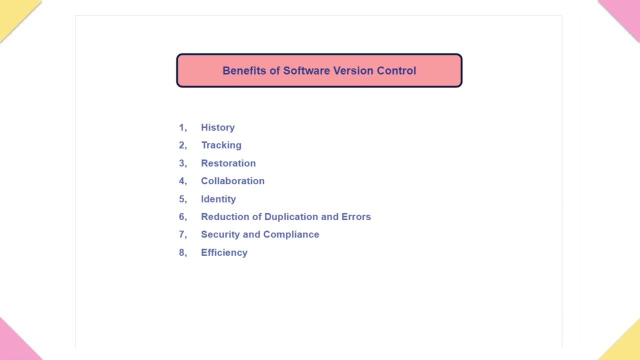 5. Identity: Identity is one of the main feature that provides authentication and authorization of developers. 6. Restoration: Restoration helps to integrate developers team to merge their source code into single project. 7. Reduction of duplication and errors: It's reduces times and reduces developer repeatable errors. 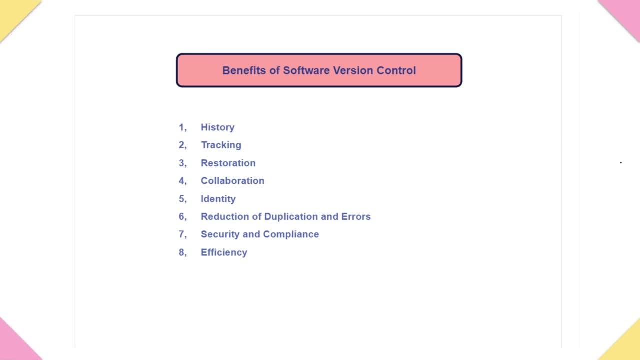 7. Security and compliance: Security is the one of the main factor that usage of software versioning control system. There is different type of tools and compliance standards are available based on the vendor and its company standards. 8. Efficiency: Using software versioning control is the one of the efficient way that managing source code of the project is possible. 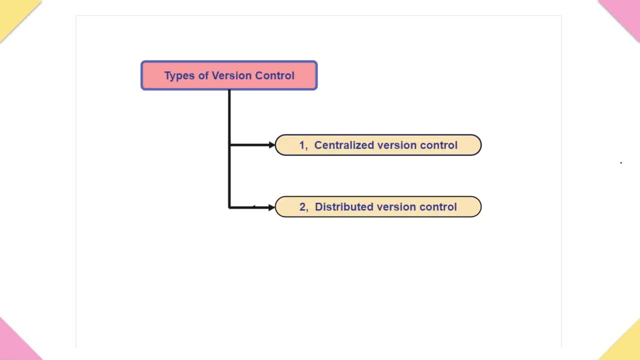 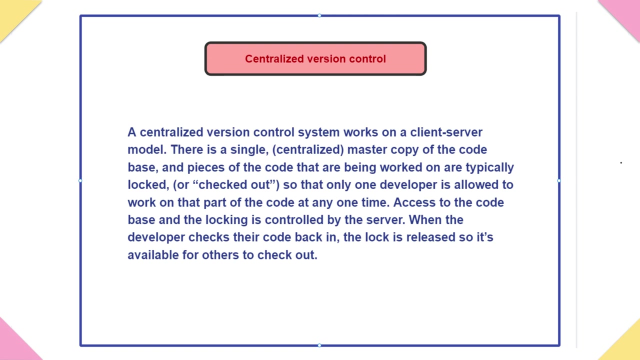 6. Restoration. There are two type of software versioning control system: 1. Centralized version control, 2. Distributed version control. Now we can discuss about centralized version control system with more details. A centralized version control system works on a client-server model. 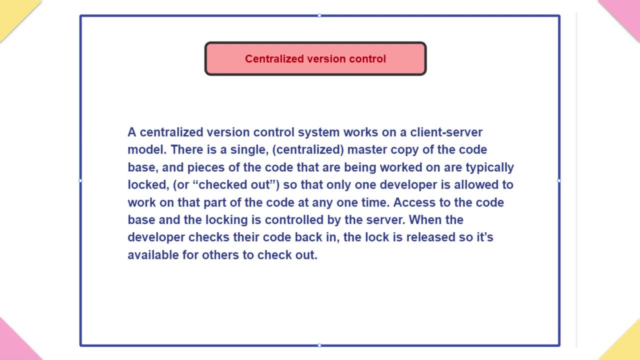 15. Present and Present На mêlе. A centralized version control system works in the context of a client-server model. There is a single centralized master copy of the codebase, and pieces of the code that are being worked on are typically locked or checked out so that only one developer is allowed to work on that part of the code at any one time. 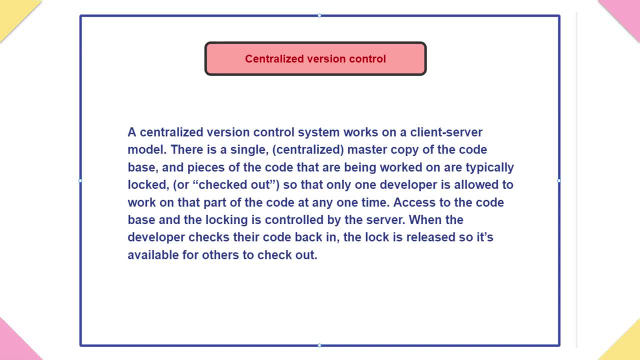 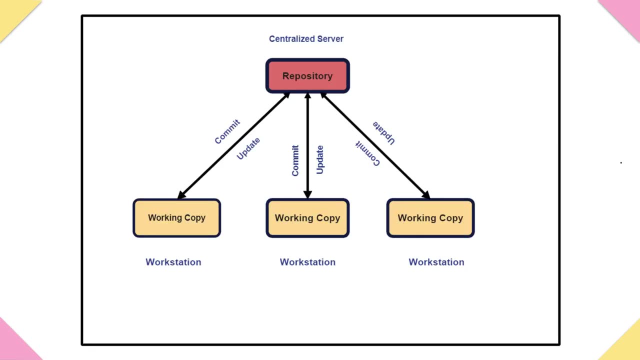 Access to the codebase and the locking is controlled by the server. When the developer checks their code back in, the lock is released, so it's available for others to check out. The following diagram would assist to understand how the centralized versioning control system works. 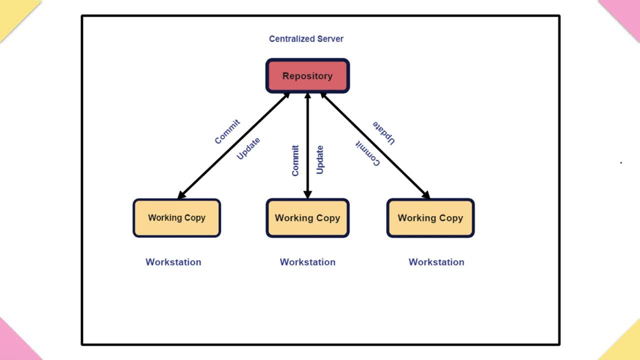 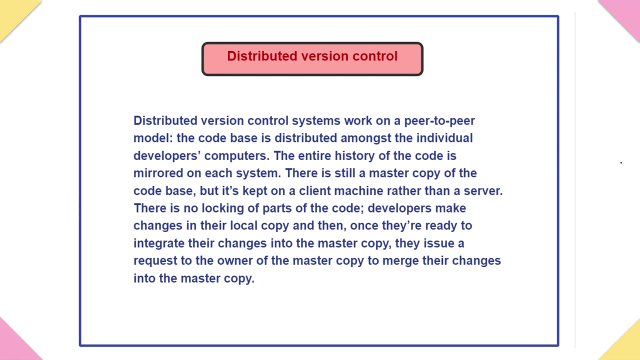 How the developer commit his source code from workstations into centralized server and updating. Next we can discuss how the software works. Next, we can discuss how the software works. Next, we can discuss how the software works. Next, we can discuss about distributed version control system with detailed information. 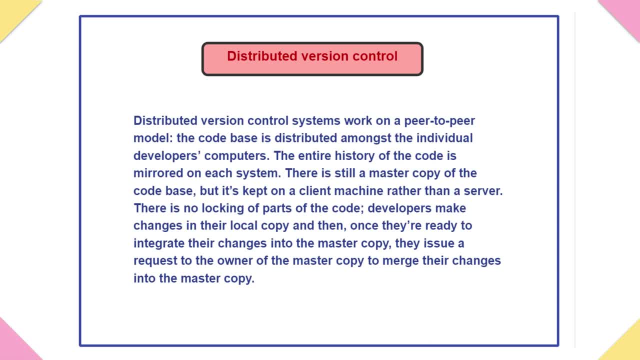 Distributed version control systems work on a peer-to-peer model. The codebase is distributed amongst the individual developer's computers. The entire history of the code is mirrored on each system. There is still a master copy of the codebase, but it's kept on a client machine rather than a server. 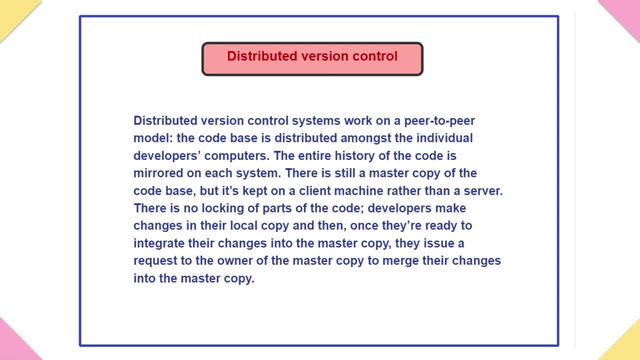 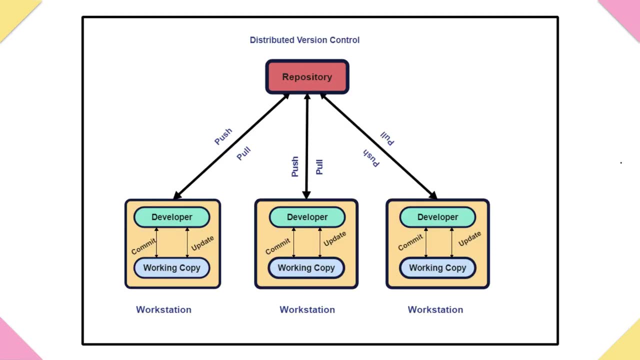 There's no locking of parts of the code. developers make changes in their local copy and then, once they're ready to integrate their changes into the master copy, they issue a request to the owner of the master copy to merge their changes into the master copy. The following diagram would assist to understand. 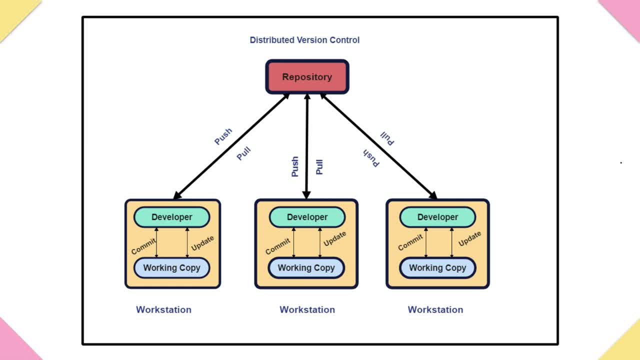 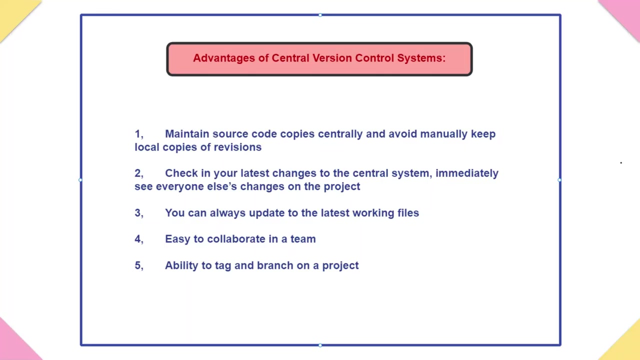 the distributed versioning control system, The developer committing source code within his workstation and there is no locking system within Workstations N with distributed version control system. Now we can discuss about what are the advantages of the centralized versioning control system. 1. Maintain source code copies centrally and avoid manually. keep local copies of revisions. 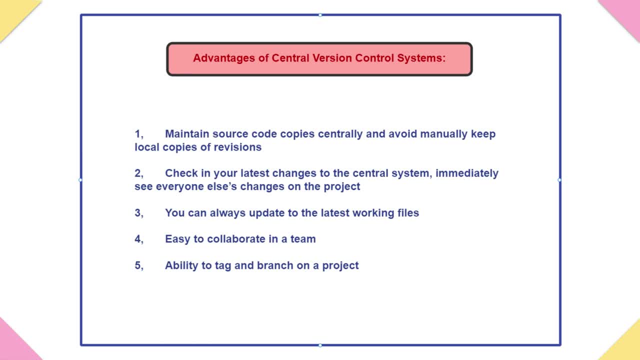 2. Check in your latest changes to the central system immediately see everyone else's changes on the project. 3. You can always update to the latest working files. 4. Easy to collaborate in a team. 5. Ability to tag and branch on a project. 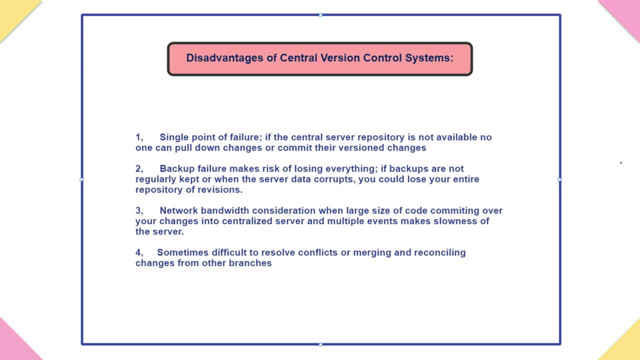 4. Easy to collaborate in a team. Now we can list some of the disadvantages of centralized version control system. 1. Single point of failure: If the central server repository is not available, no one can pull down changes or commit their version changes. 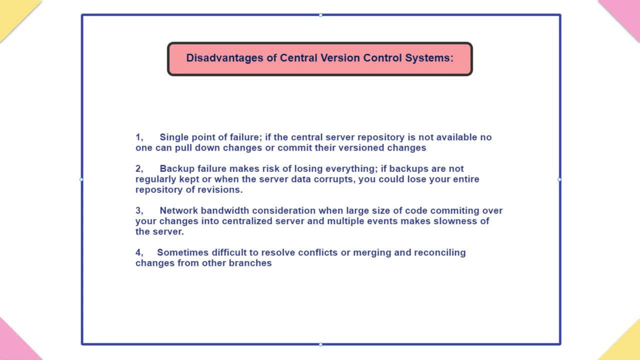 2. Backup failure makes risk of losing everything. If backups are not regularly kept or when the server data corrupts, you could lose your entire repository of revisions. 3. Network bandwidth consideration when large size of code committing over your changes in decentralized server and multiple events makes slowness of the server. 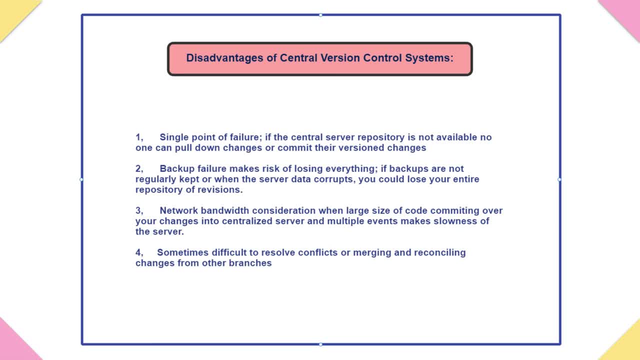 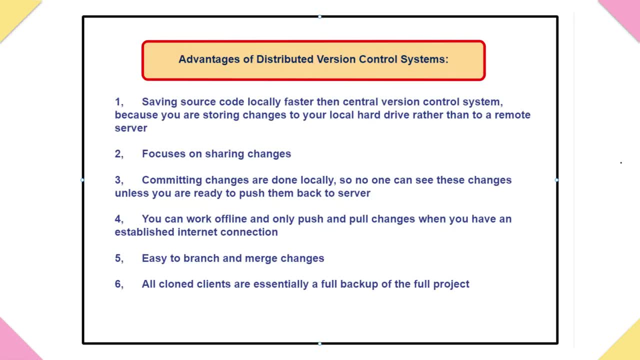 4. Sometimes difficult to resolve conflicts or merging and reconciling changes from other branches. Next we can discuss that. what are the advantages of distributed version control systems? 1. Saving source code locally faster than the server. 1. Saving source code locally faster than the server. 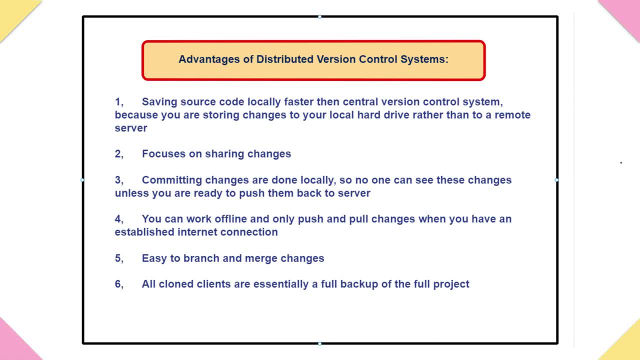 1. Saving source code locally faster than the server. 1. Saving source code locally fast than the server. 1. Saving source code locally faster than the server. 1. Saving remote server. 1. Saving remote server. 1. Saving resources more quickly than between oneself and the backup server, such as network. 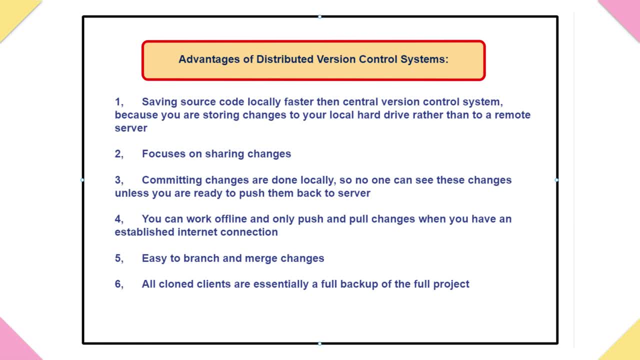 Information Pack: 2. Increasing més frecuis. 1. Increase storage complexity. 2. Increase storage. LGBTQI vulnerability: 1. Increase more storage complexity. 1. Increase storage complexity. 2. Increase sharing diversity: 1. Increase and sharing sharing diversity. 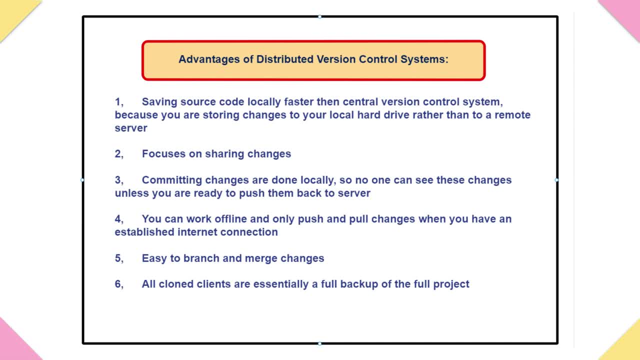 MERP: 1. Increase the size of chips and Yummy, over about 500 thousand hits hurt that setup. 3. Increase reliable. Então eu possoopt argentês, você vai onde remover mais barraMa+. So added in porting colleagues to the results of the freepoint management process: 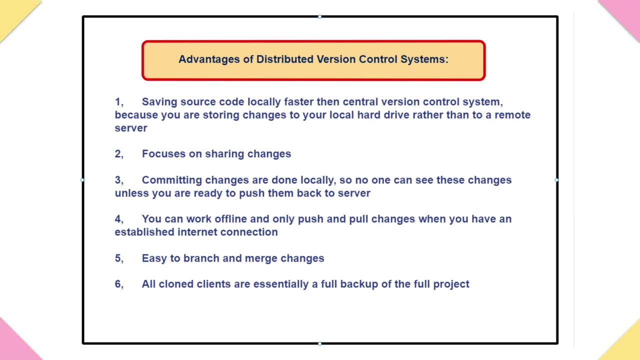 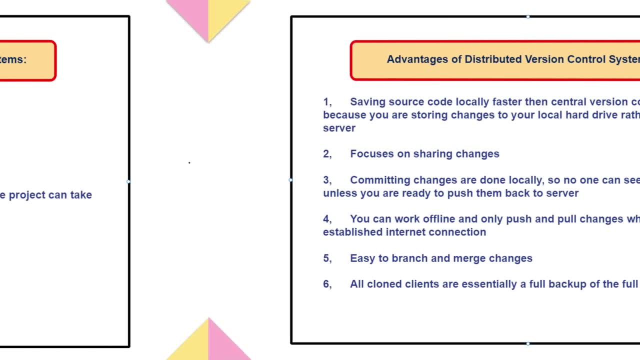 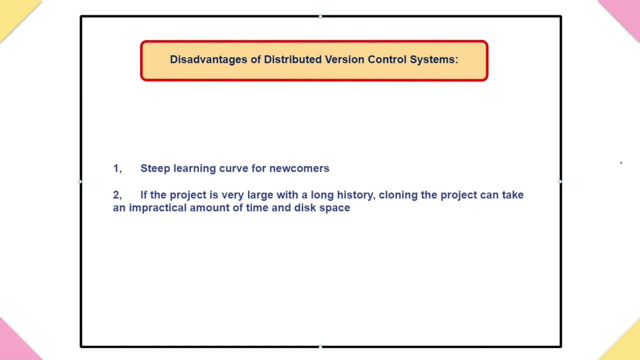 ださい舐 to branch and merge changes. six: all cloned clients are essentially a full backup of the full project. let us discuss about disadvantages of distributed version control systems. one: steep learning curve for newcomers. two: if the project is very large with a long history, cloning the project can take an impractical amount of time and disk space. 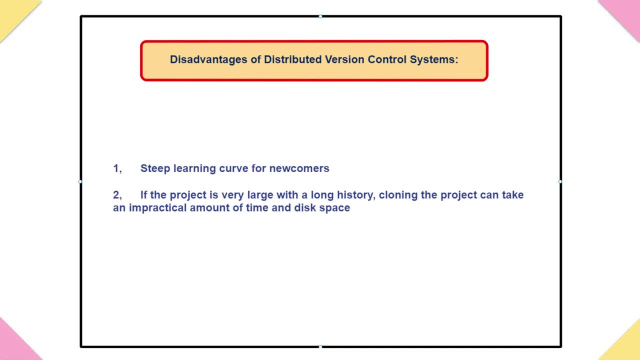 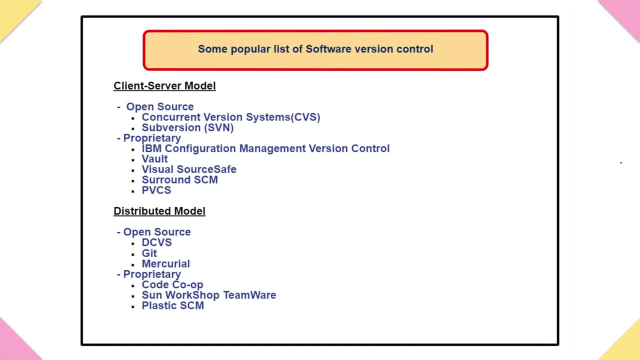 there are some popular tools are available on the market and internet portal. two types of tools. one is open source and another one is proprietary. on each centralized version control system and distributed version control system, few popular tools can be list here: open source under client server model, concurrent version systems, cvs, subversion, svn. under proprietary.